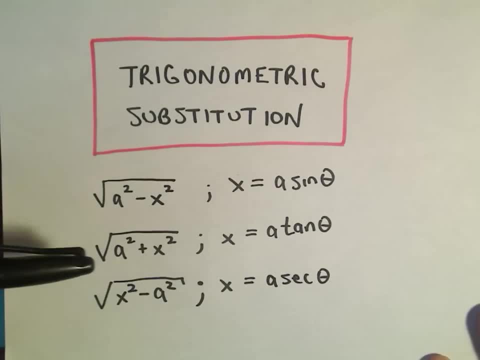 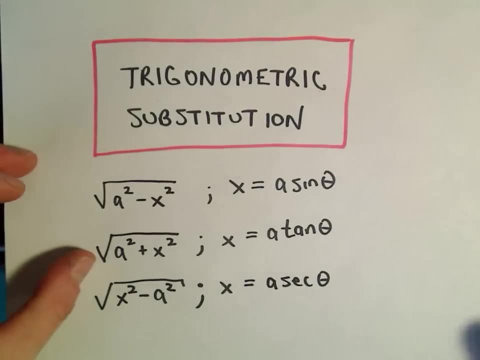 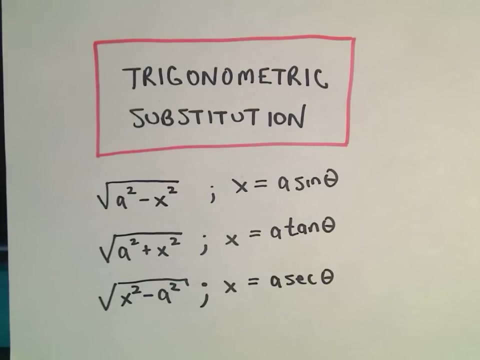 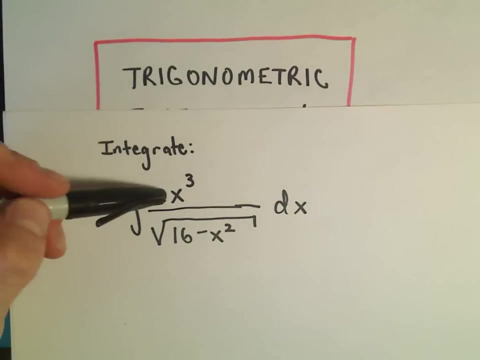 Plus a variable squared, or a variable squared minus a number squared. Notice, there's no, you know, x to the first power in here. If there is a term involving x, we're going to have to actually do completing the square and it's going to get a little bit more involved. We'll do that in a different example. Okay, so, depending on the form, we use different substitutions, So let's just jump in and try to do one here. So here we're going to integrate x cubed over the square root of 16 minus x squared. 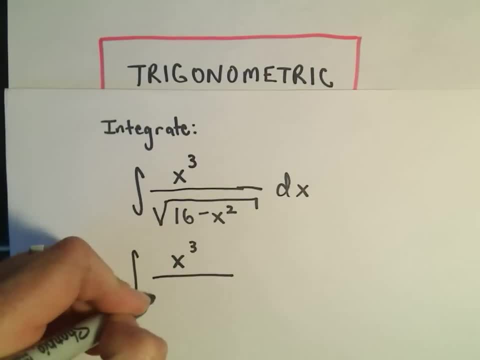 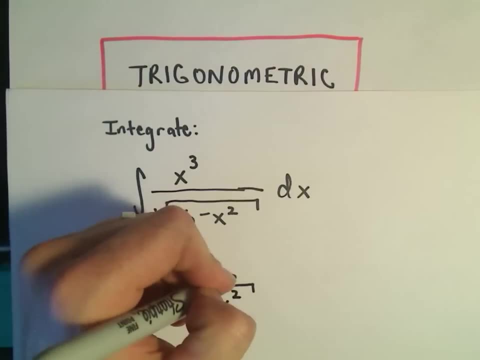 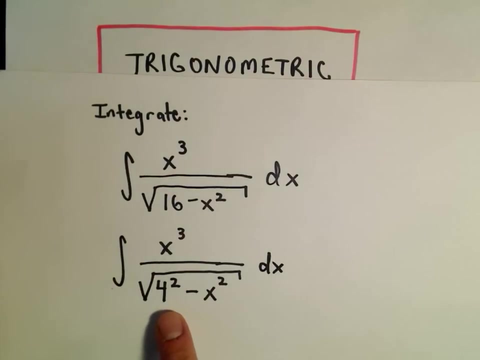 The first thing. I mean you don't really have to do this. I'm going to do it just to try to make it explicit here: 16. we can write that as 4 squared, Well, minus x squared, And then our dx is left hanging out. So our radical, the square root that I'm trying to somehow deal with, notice there's a, the number comes first and then we're subtracting a variable. 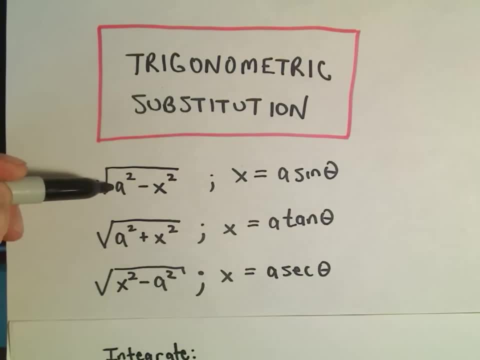 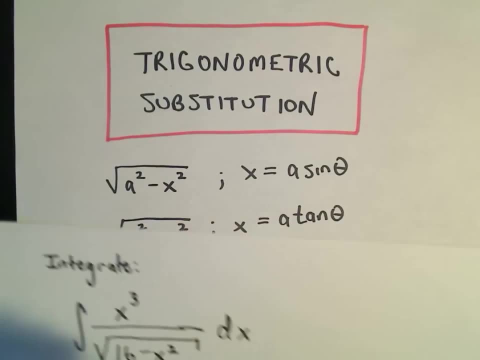 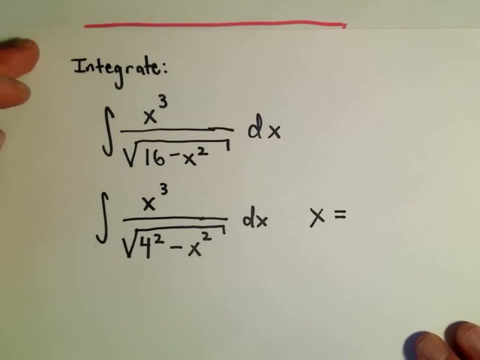 Well, our very first type of substitution. it says: if you have a number being squared Minus a variable being squared, It says we're going to use the substitution x equals. and then it says, basically, take whatever number is being squared. So in this case the number being squared is 4.. So we're going to use the substitution x equals 4 sine theta. 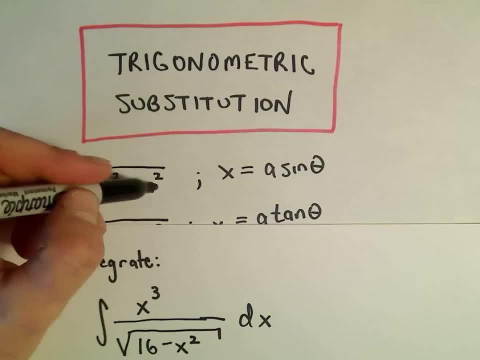 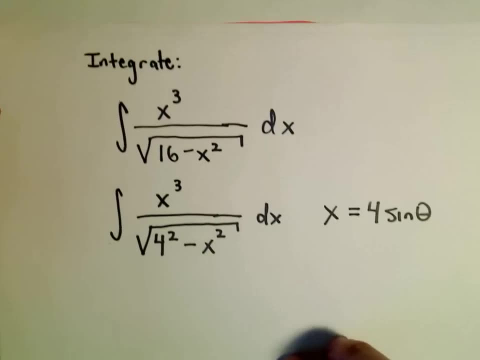 So again, depending on you know the type of quadratic underneath the radical, you use different substitutions And in a second you'll see we'll use a trig identity and that's going to make everything go away. So that's going to be kind of the point of all this. 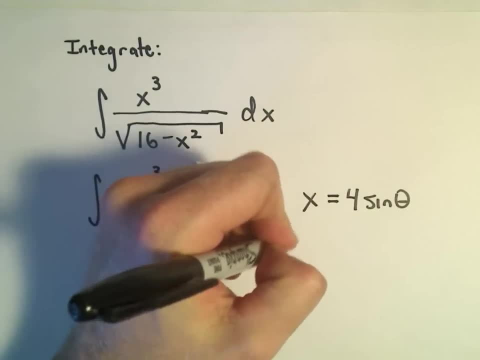 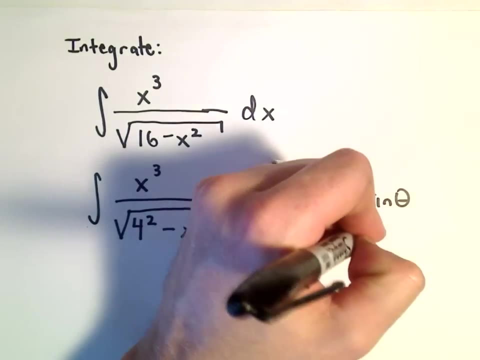 All right, a couple things. x is 4 sine theta. From that we can compute our dx value. We're just taking the derivative of the right side. Well, we'll get 4 cosine theta, d theta as. and really you're doing a differential here. 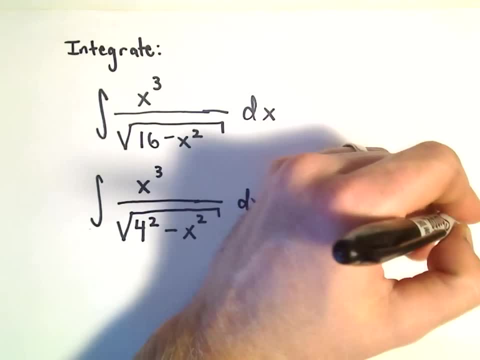 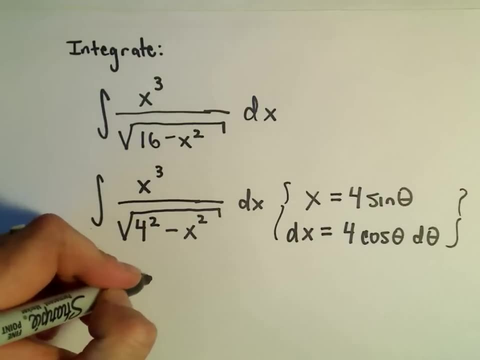 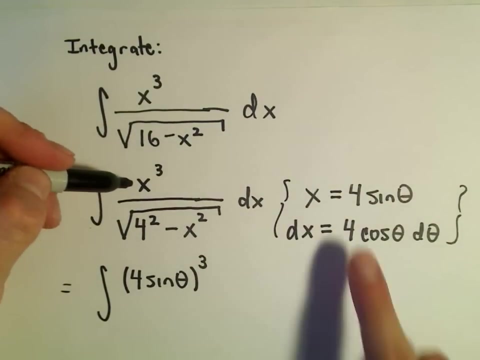 So now I'm just going to simply use all of this stuff. I'm going to substitute This into my equation, simplify it down and hopefully it won't be a big ol' mess to integrate. So let's see, We've got 4 sine theta cubed. I'm just plugging in that my x is 4 sine theta. 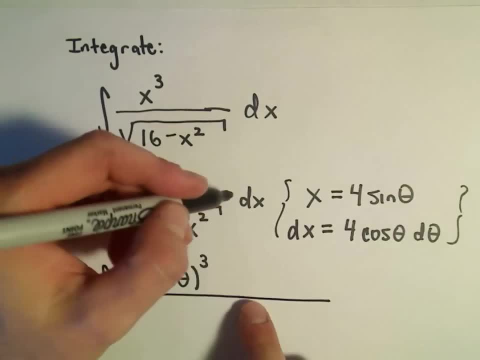 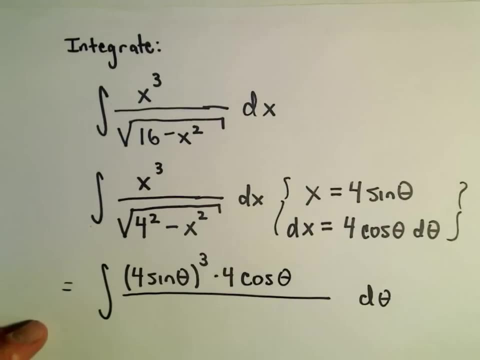 We've got our dx hanging out over here on the right. I'm just going to plug my dx- Imagine it's in the numerator. So we'll have 4 cosine theta and I like to put my d theta over to the side. 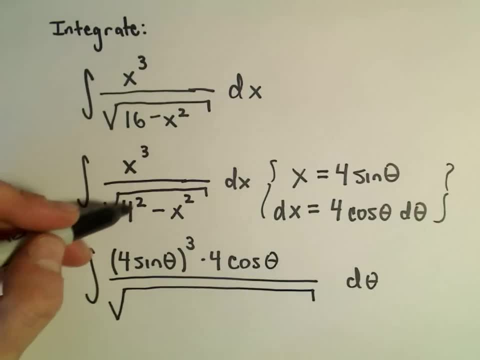 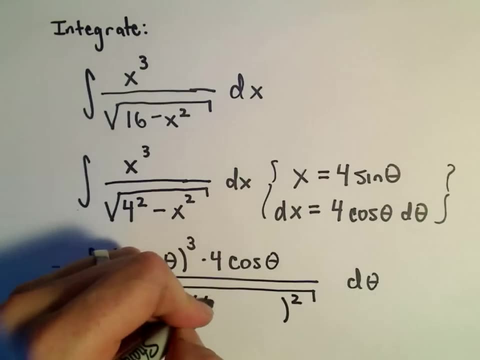 Underneath our square root. I'm going to go back and write this 4 squared, I'm going to put it back as 16. And then we've got minus x squared. But again, I'm just plugging in that x is 4 sine theta. 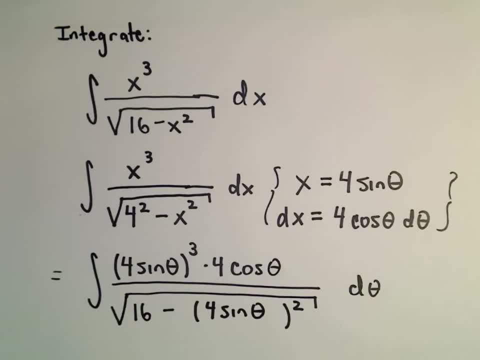 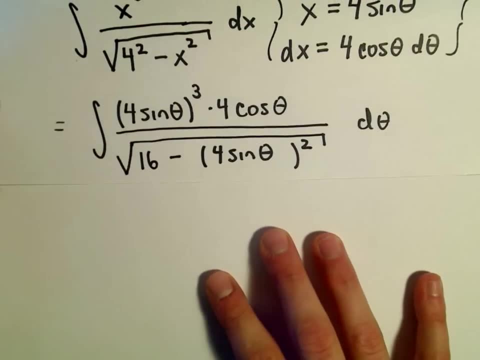 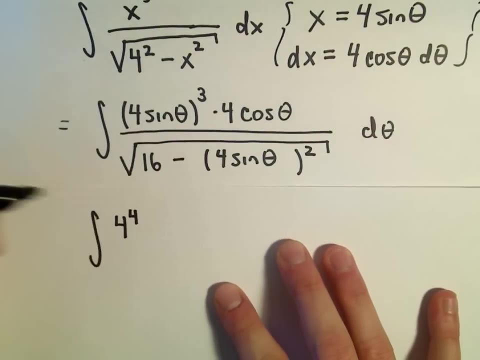 Okay, so that's the first part. Nothing, you know, nothing crazy. It's just again kind of remembering the correct substitution to use, And now we have to try to integrate this lovely thing. All righty. so let's see, We've got 4 cubed times, another 4.. That's going to give us 4 to the fourth. 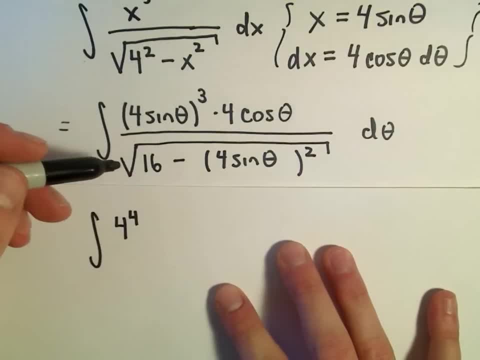 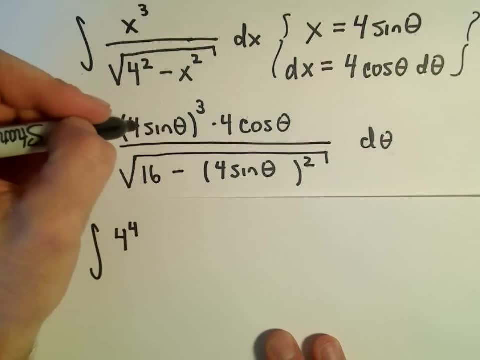 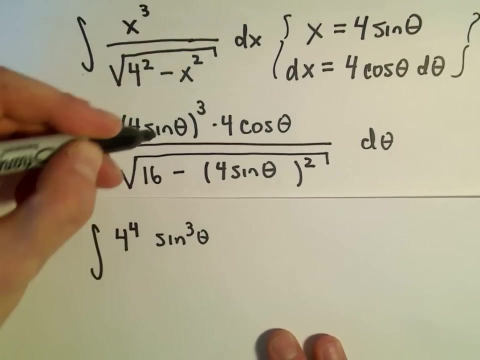 I usually don't multiply them out because you'll end up picking up constants in the denominator and hopefully things will cancel. So, just being a little bit- I was going to say lazy, but probably efficient is a better word- We've got 4 cubed times 4, which is 4 to the fourth We would have sine cubed theta when we cube. 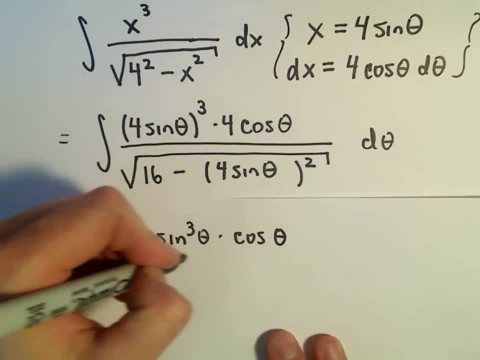 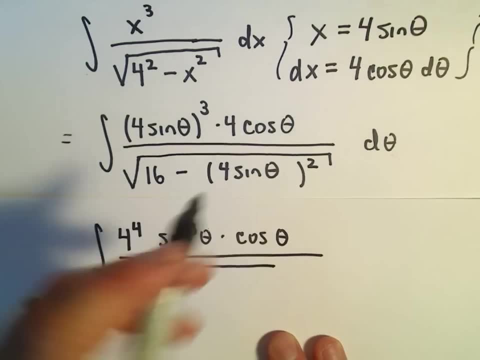 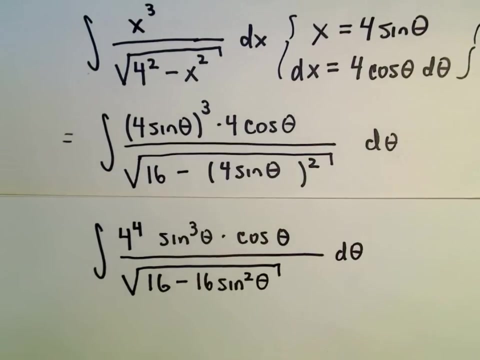 Cosine theta- he's just still just hanging out- And the denominator. well, we've got 16 minus. If we take 4 sine theta and square it, that'll give us 16 sine squared theta And again d theta just hanging out. 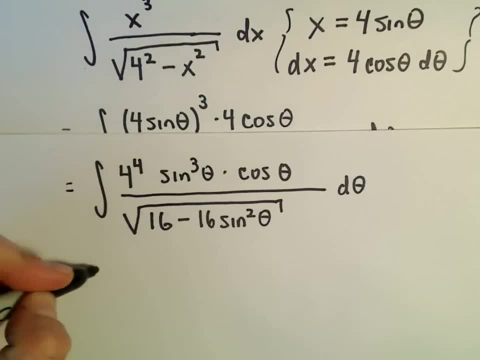 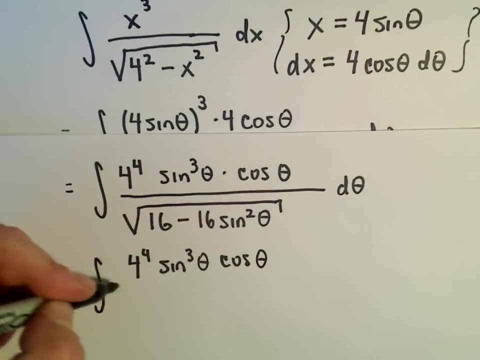 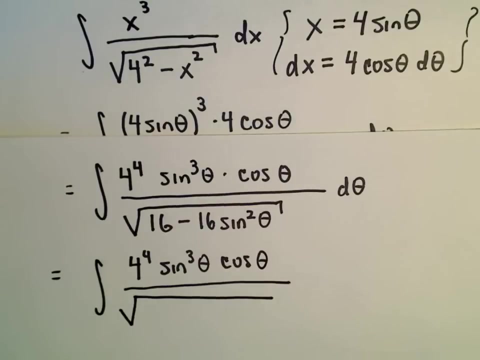 Let's see. And now again, just keep simplifying is all we're doing here. So 4 to the fourth- I'm not doing anything in the numerator And this is kind of the magic. Notice the coefficients. They both have 16s, which is what you want. 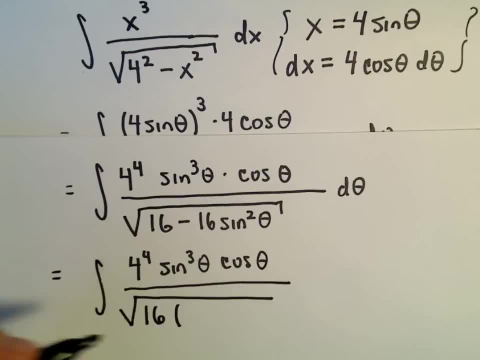 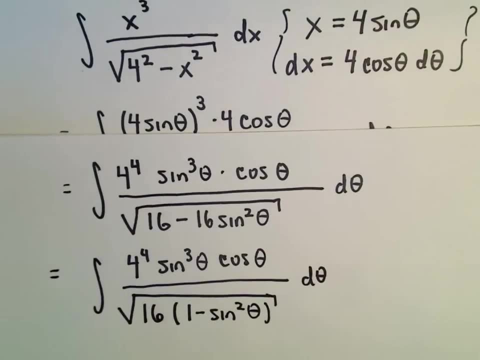 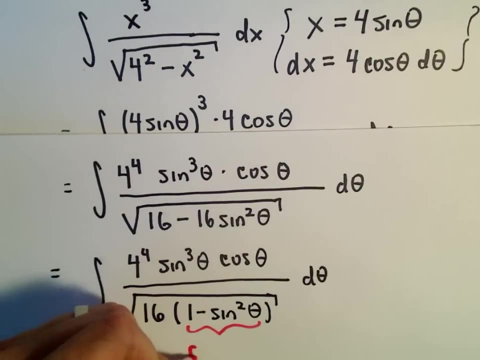 Because we can factor that 16 out, It's still underneath the radical. We would have 1 minus sine squared theta, And now- this is the point, though- We can use our trig identity on 1 minus sine squared theta. That's simply going to be the same thing as well. cosine squared theta. 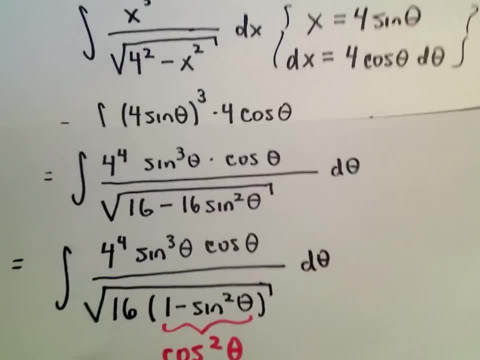 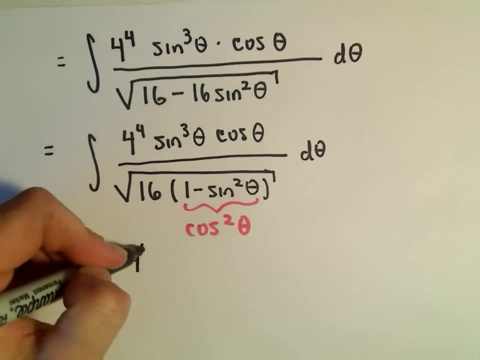 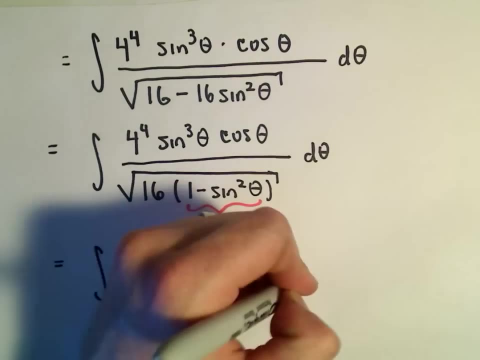 And this is a good thing. We're making everything underneath the square root. We're going to make it be a perfect square, All right. So we've got 4 to the fourth. We've got sine cubed theta, cosine theta. 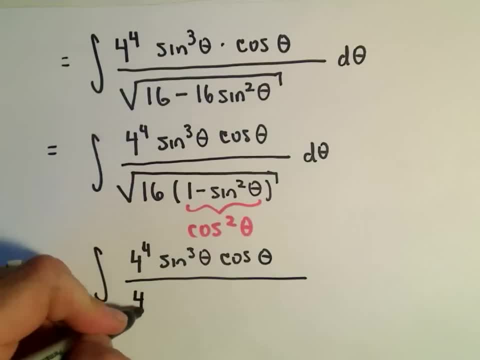 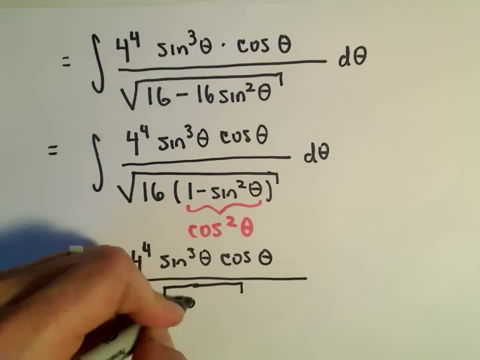 Okay, So we can take the square root of 16. That would just give us, well, 4.. And again, we're going to replace the 1 minus sine squared theta with cosine squared theta. Then we still have our d theta left over. 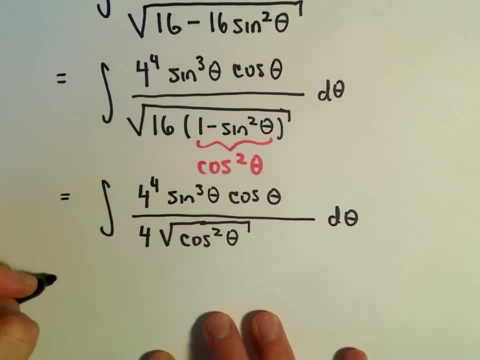 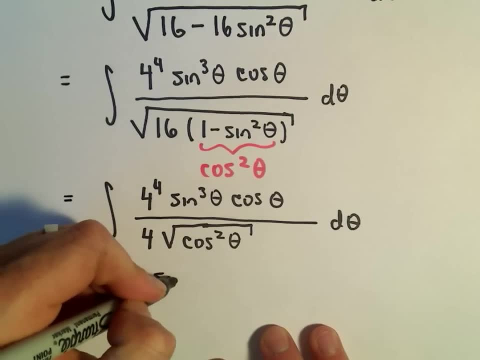 And again, we're just going to keep simplifying here a little bit further. Okay, So 4 to the fourth over 4 to the first will be 4 to the third. I'm just going to pull that out front. We still have sine cubed theta, cosine theta. 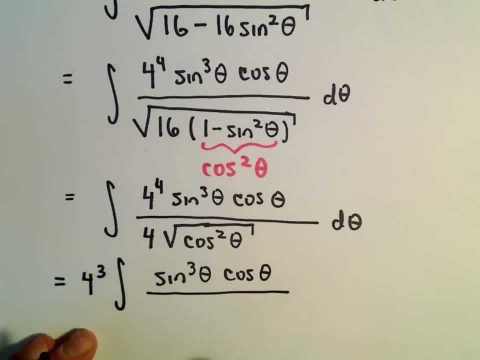 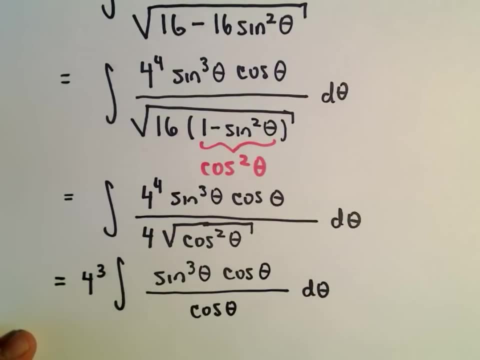 And again in the denominator. now, well, if we take the square root of cosine squared, that's going to give us cosine theta. And lo and behold, we have now gotten rid of our square root. So that's kind of step one to me. is just getting to this point. 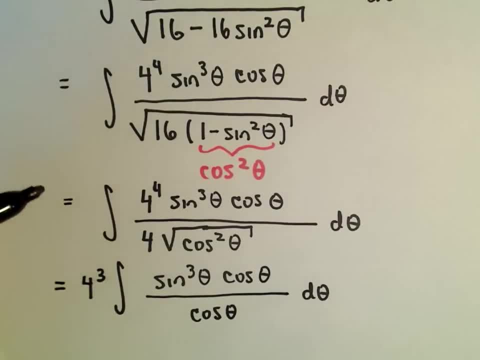 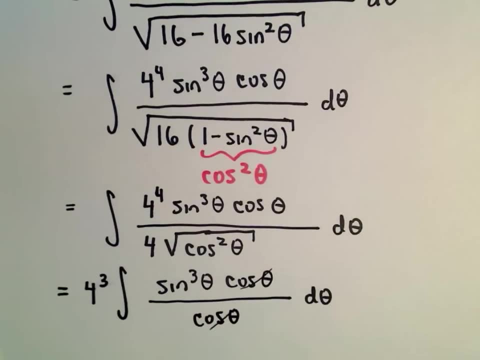 Now you have a lovely trigonometric integral And these can be relatively easy or a little more involved to integrate, So I'm just going to cancel out the cosine thetas here. So really we have turned this problem into integrating 4 to the third. 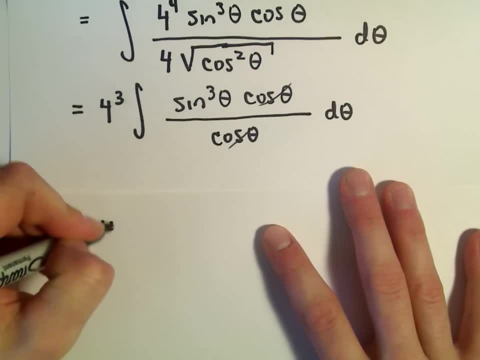 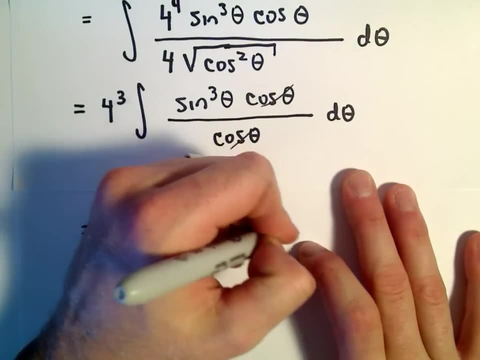 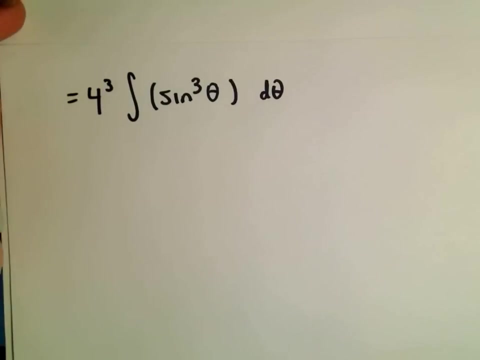 Again, you could multiply that out 4 to the third And we would be left with sine cubed theta, d theta. Okay, So now the question is: well, how on earth do you integrate sine cubed theta So typically in a calculus class? you should have seen trigonometric integrals before this. 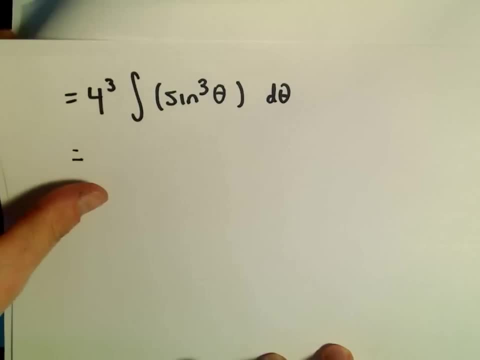 And kind of the trick. on this one there's, you know, some hints or some tricks. One of the tricks is if you have an odd power of sine or cosine, a lot of times what we'll do is we'll break that up. 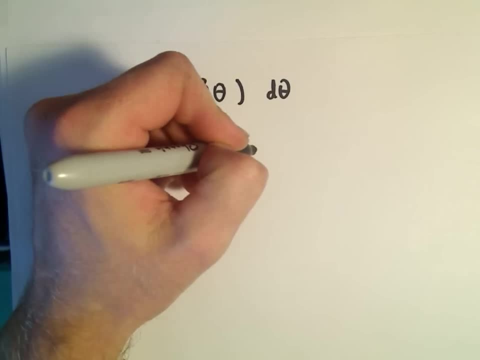 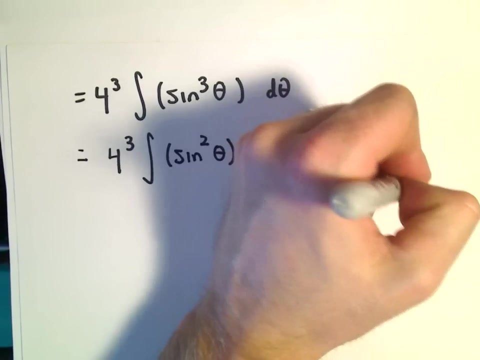 So I'm going to write this as sine squared theta times, sine theta d theta, And again, what we're going to do is we're going to use our trig identity. So, cosine squared theta Plus sine squared theta, That equals 1.. 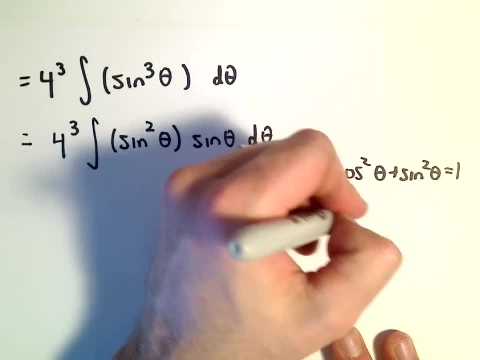 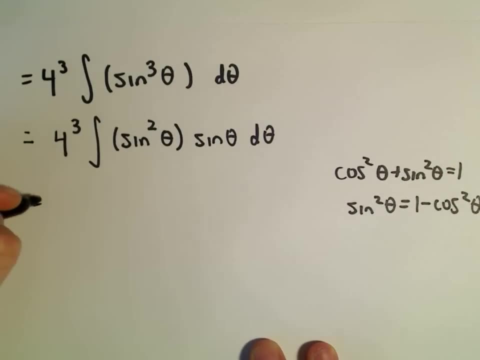 Whoops, let's squeeze that in there. So equivalently. well, sine squared theta is just going to be 1 minus cosine squared theta, And that's what I'm going to plug in. So we've got 4 to the third. 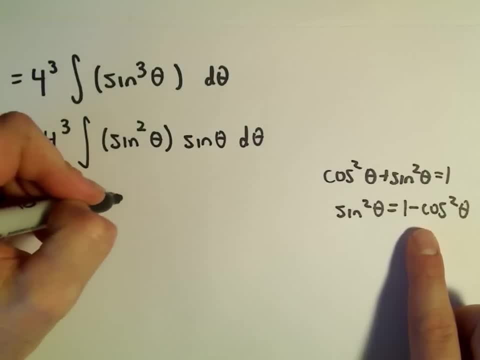 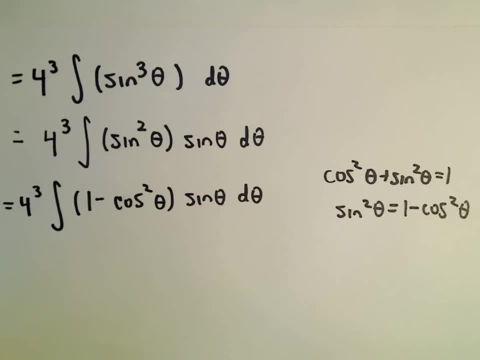 I'm going to replace my sine squared with 1 minus cosine squared theta, And then we still have sine theta left over. And well, you know why on earth would we do this? We do this because we're going to make a? u substitution work. 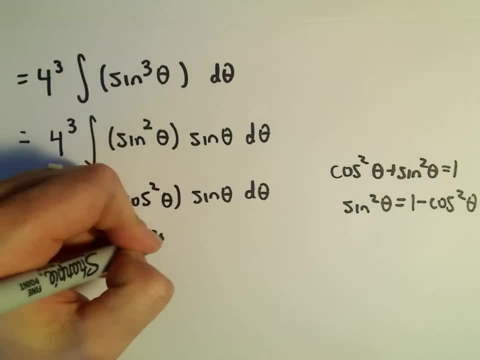 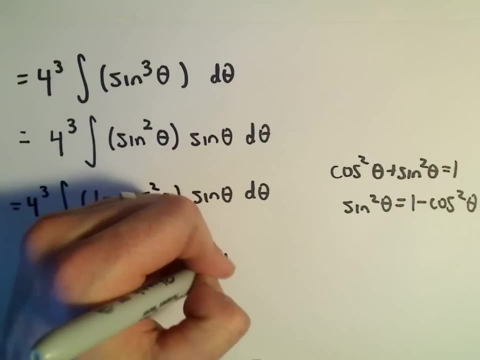 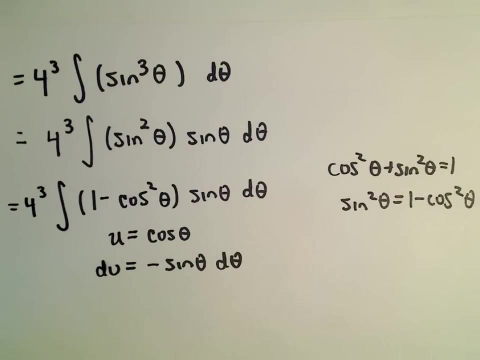 So we can let u, in this case, simply equal. well, just plain old cosine theta du would be negative sine theta d theta. Well, we don't have a negative sine theta d theta, We have a positive sine theta d theta in our problem. 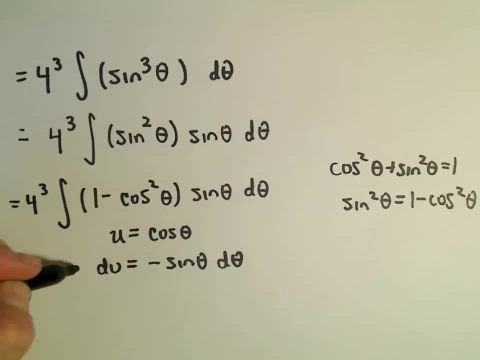 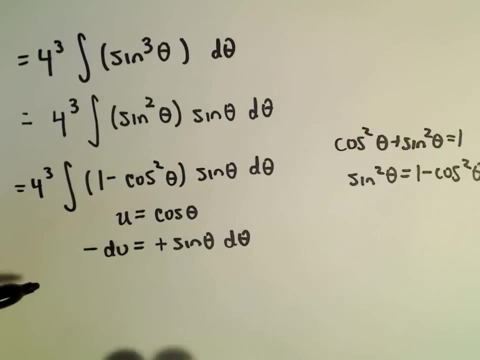 So I'm just going to multiply both sides of my du equation by negative 1.. So I'll have negative du on the left And then that would turn into positive sine theta d theta on the right. All right, so, as you can already see, these are long problems. 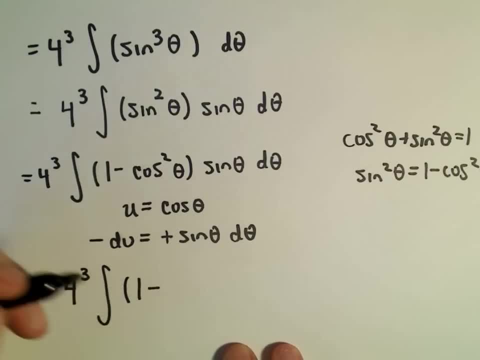 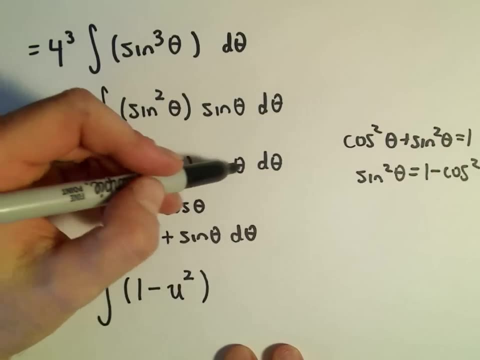 So 4 to the cubed. he's still hanging out. Notice, now we have 1 minus. well, cosine of theta, That's what we're calling u, So that will just be. u squared Sine theta, d theta, that's the same thing as negative du. 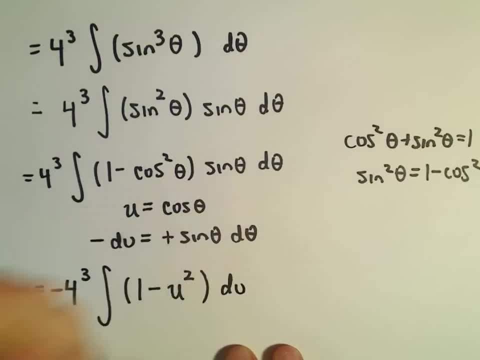 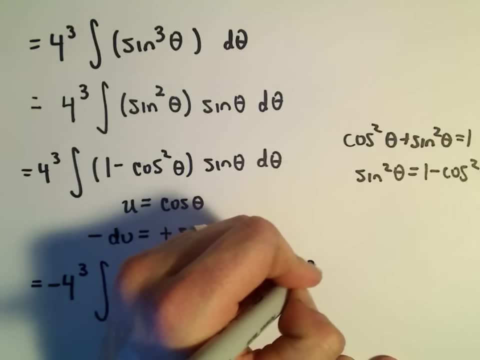 I'm going to pull the negative out front And hey, there's my du. And now this is easy to do, Now this is easy to integrate. This is just a polynomial. So we've got negative 4 to the third. 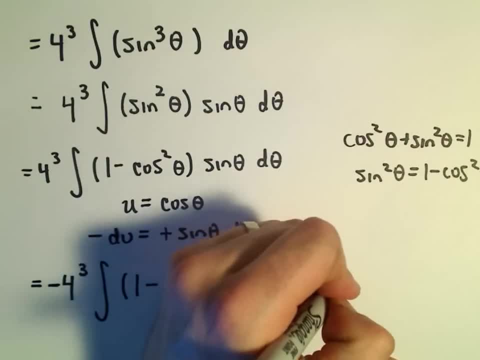 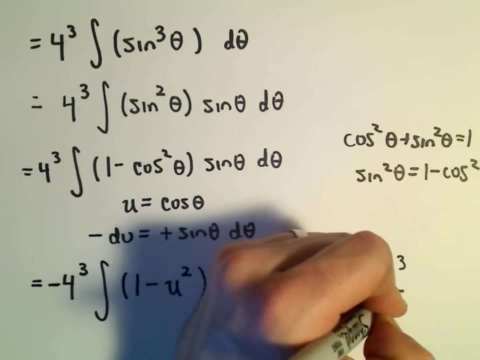 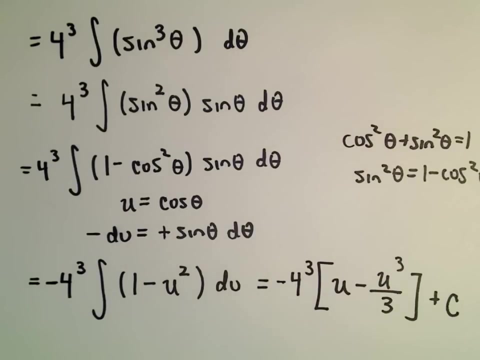 The antiderivative of 1 with respect to u would simply be u, And then we would have: when we integrate u squared, we'll get u cubed over 3 plus c. OK, so now we've got to start backtracking right, because our original problem involved x, not u. 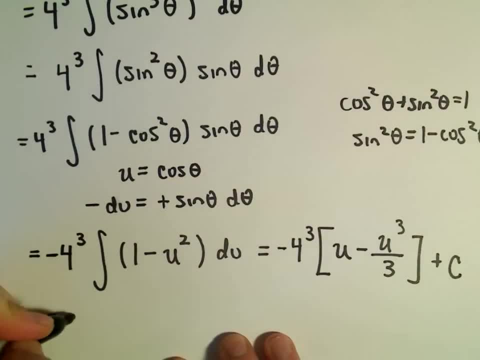 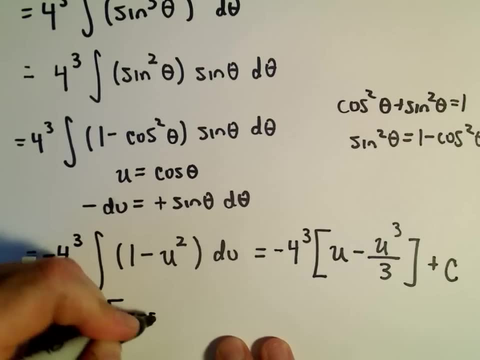 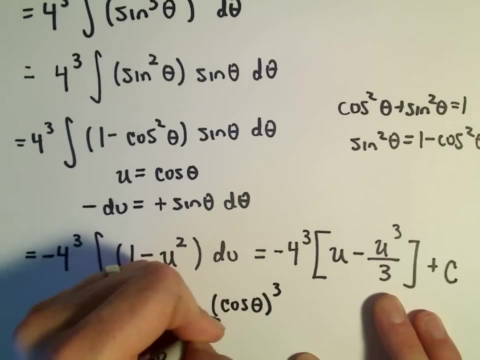 So we'll have to start backtracking. So we've got negative 4 to the third u. we said that's the same thing as cosine theta. So then we've got cosine theta minus cosine theta cubed over 3 plus c. 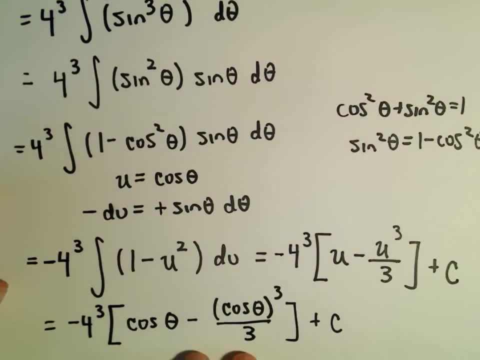 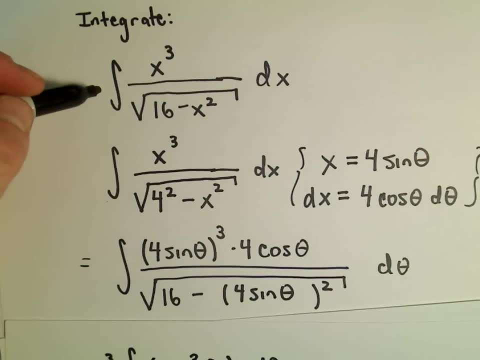 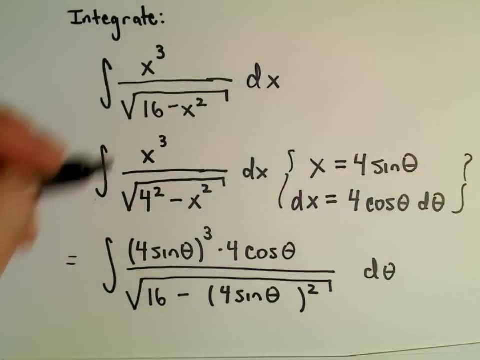 OK, now we're still not done yet, because our solution here involves theta, But again, our original problem involved x. Remember this was the very original thing that we were trying to integrate, So we have to somehow now go from thetas back to x's. 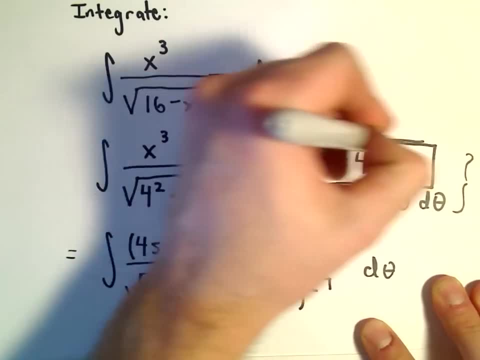 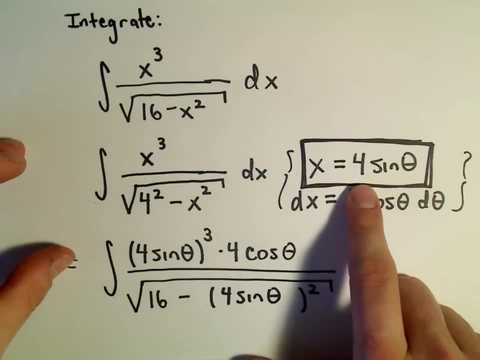 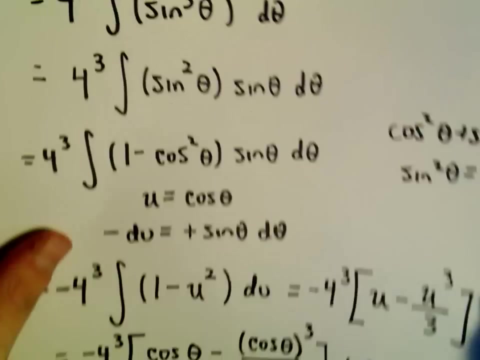 And it all comes back to this very original, you know, substitution we made to get the ball rolling, So here's how we do it. So, OK, we used x equals 4 sine theta. That was our substitution, So I'm going to make a little note of that. 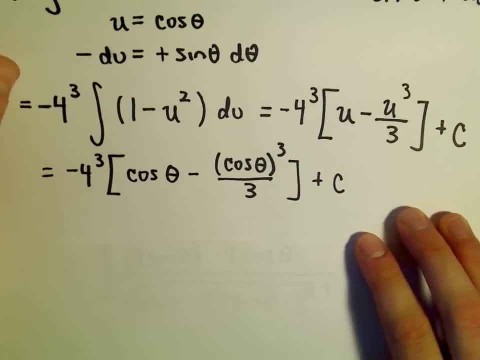 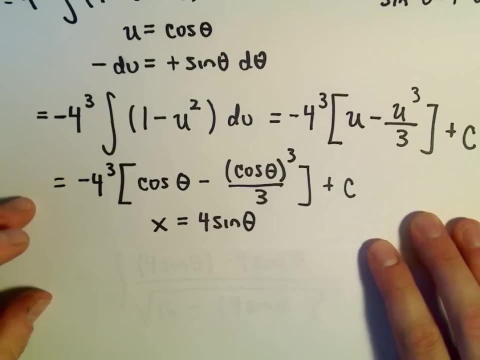 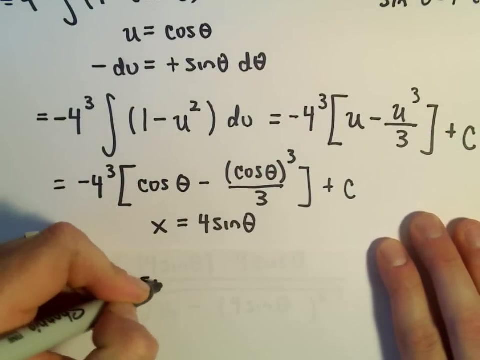 Let me grab some more paper here. OK, so we used the substitution x equals 4 sine theta. What we do is we make a little right triangle. I'm going to divide both sides by 4.. So that would give me simply x over 4 equals sine theta. 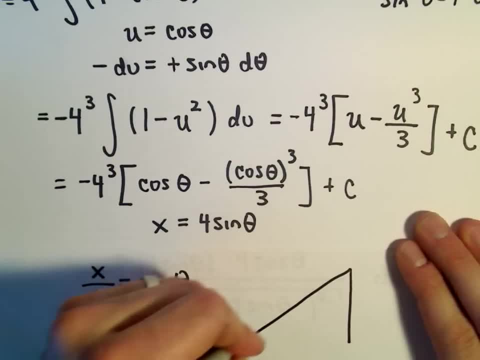 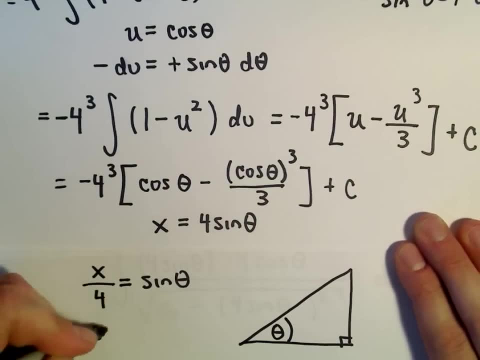 And now I'm going to make a little right triangle based on this. So here's going to be my angle: theta, Remember SOHCAHTOA, SOHCAHTOA. So remember sine of an angle That equals the opposite side divided by the length of the hypotenuse. 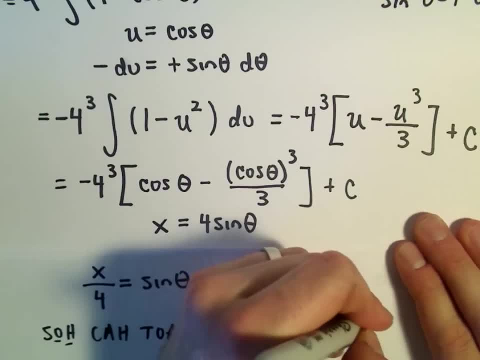 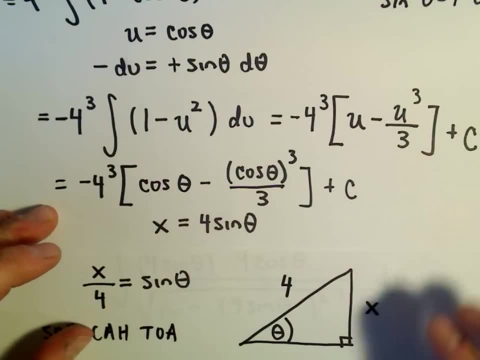 So the opposite side, that's the numerator, We can just simply say that that's x, The hypotenuse, we can say that that has value 4.. And if we do Pythagorean theorem to figure out the missing side, So the missing side squared plus x squared. 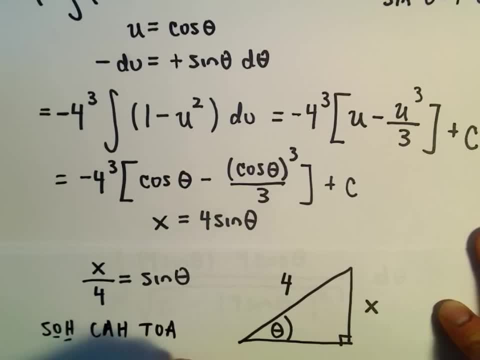 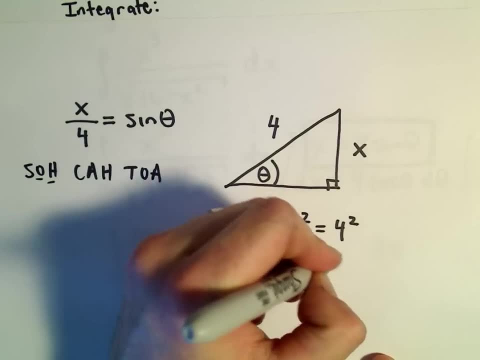 Equals 4 squared, If you solve for the missing side here. So if you solve for the missing side here, We'll simply get: 4 squared is 16.. We'll subtract the x squared. We'll take the square root of both sides. 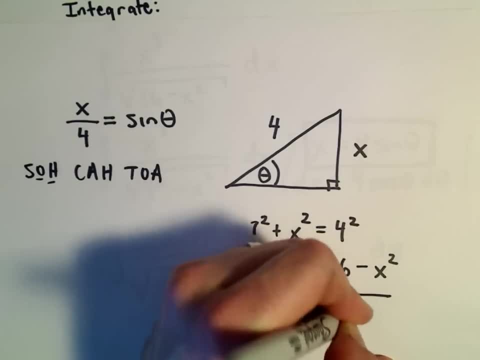 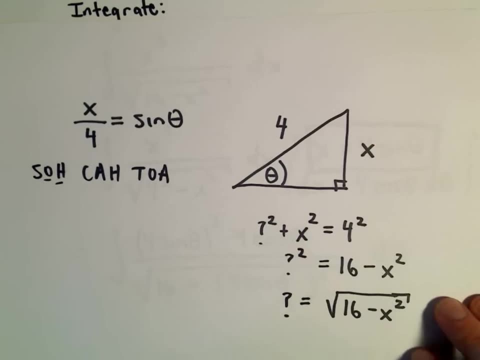 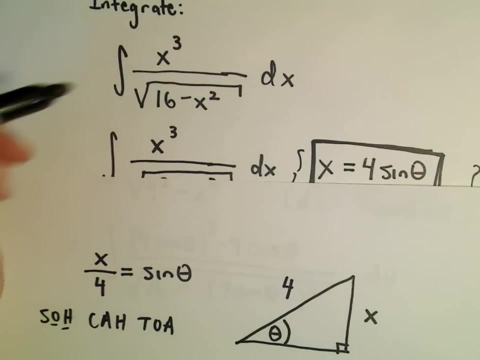 And we'll get that. the missing side is the square root of 16 minus x squared. OK, Notice in the very original problem. I hope lower is yet. Hey, that happened to be the square root we were trying to get rid of. 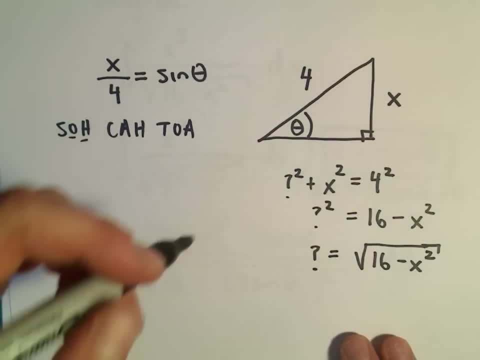 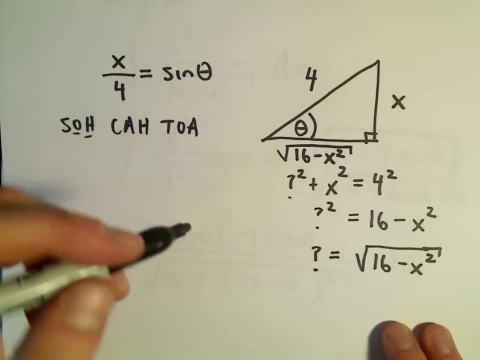 And that ended up being the missing side. So that will happen a lot of times. So, alright, I want to say always. I can swear, though at some point in my existence I saw an example where it wasn't exactly the original radical you're trying to get rid of. 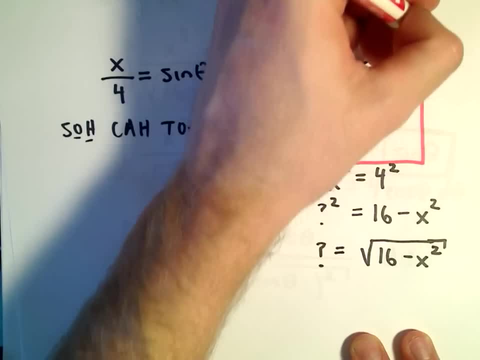 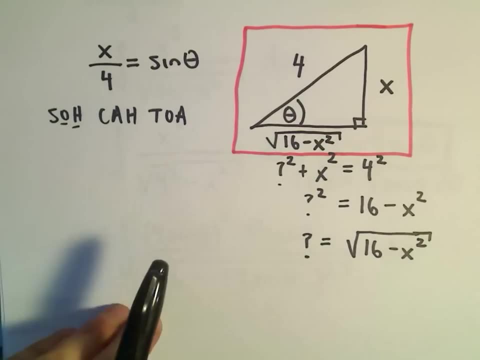 But 99% of the time at least, it seems like that's what happens. Maybe it always happens and I'm crazy and don't remember. So, OK, We're almost there, Let's go back here. OK, So now we're in business. 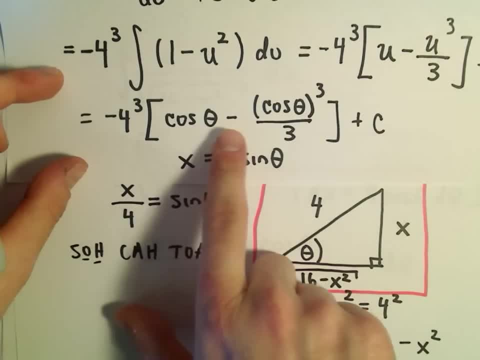 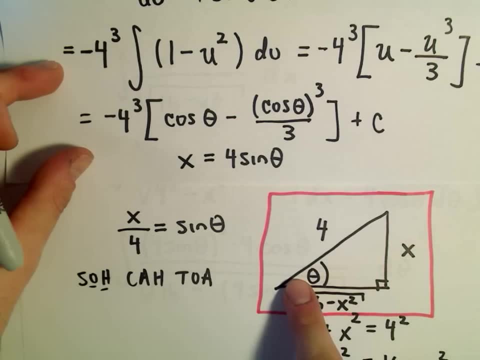 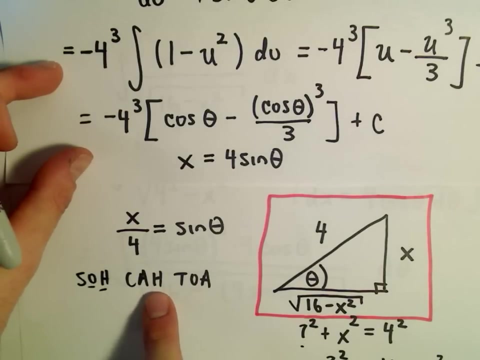 We're almost there. Our solution was negative, 4 to the third cosine, theta minus cosine theta cubed over 3 plus c. But again now the point is, by filling in this triangle I can read cosine of theta from the triangle. So remember, cosine is defined to be the adjacent side divided by the hypotenuse. 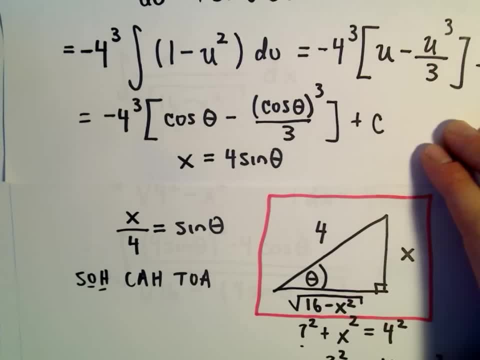 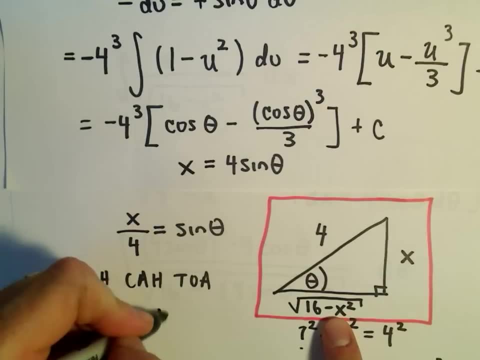 So, really, what we're going to get here, We've got the cosine of theta from my triangle. Again, it's going to be the adjacent, Which is the square root of 16 minus x squared over the length of the hypotenuse, which is 4.. 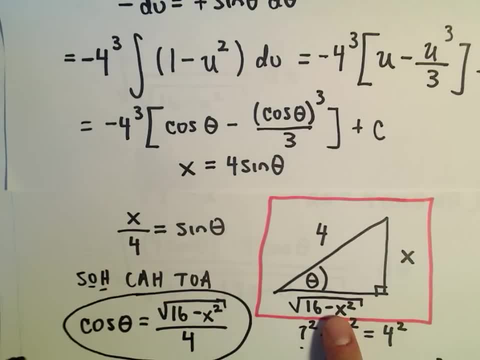 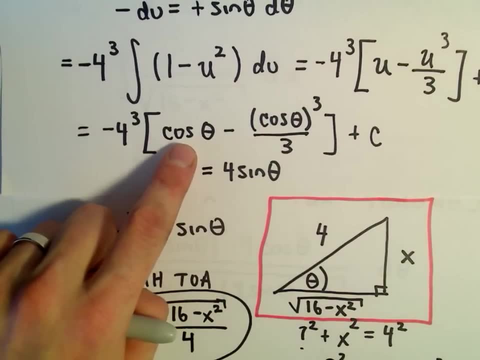 So now we've done this little right triangle trick, That's what I'm going to plug back into, Plug back in for cosine of theta And, lo and behold, We will finally have Our solution. So let's see if I can't get everything in here. 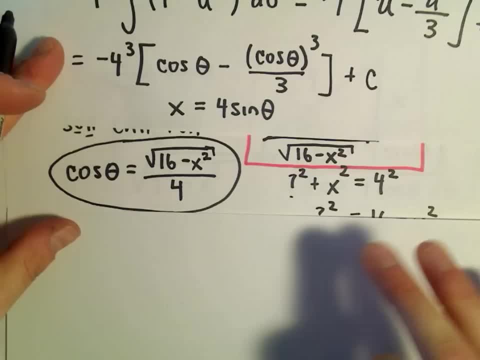 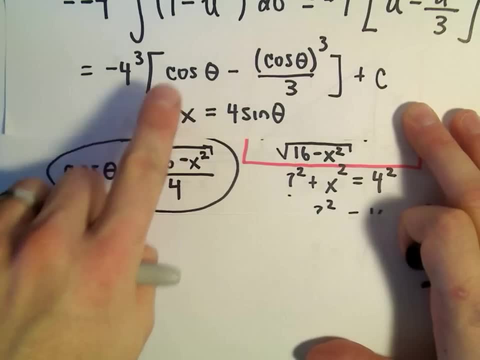 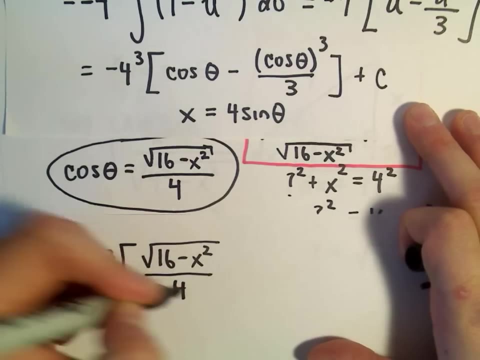 I think we can. OK, So now we're there. So we've got negative 4 to the third. Again, you can simplify that if you want to. Cosine of theta, We said that's just going to be the square root of 16 minus x squared over 4.. 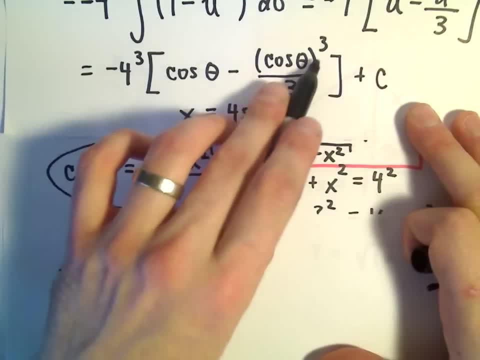 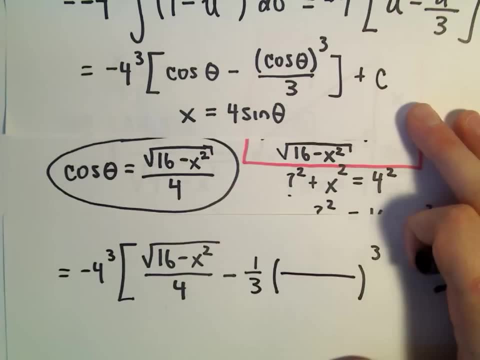 Minus. OK, We had cosine theta cubed over 3.. I'm going to pull the one third out front And then we've got cosine theta cubed. But again, we just said that cosine of theta was the square root of 16 minus x squared. 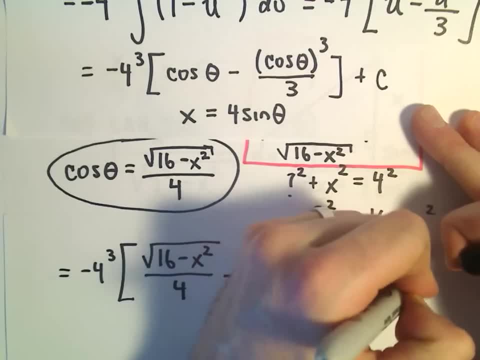 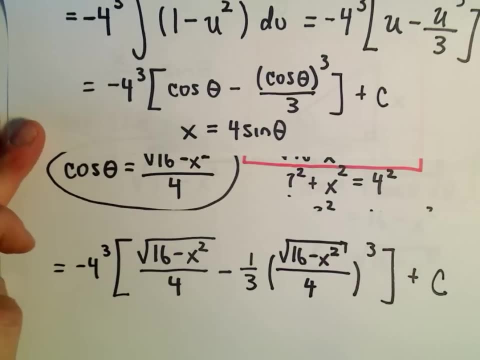 All over 4.. And now we've got our plus c still left over And, hallelujah, We've got our solution. So trig substitutions to me are long. You've got to do the substitution. You have to do the algebra. 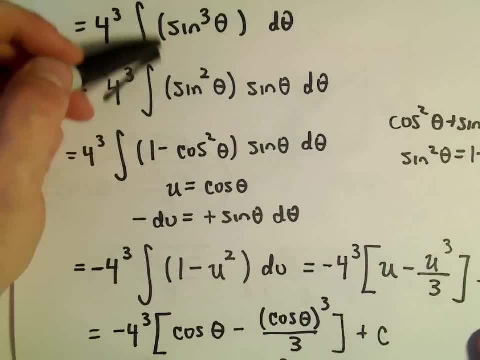 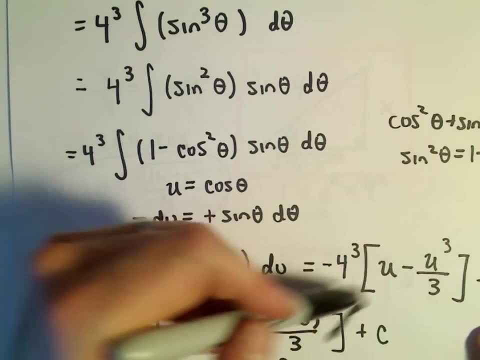 Then it turns into a trig integral that we saw here. You've got to remember how to do trig integrals, Which can be a little tricky, I think, And then you just have to basically do again this little right triangle trick To help recover the original variable.